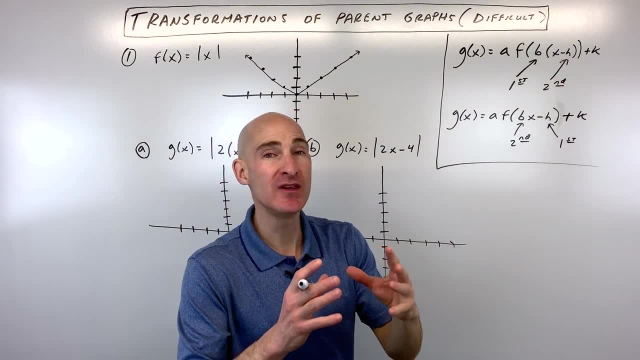 orada. so what i mean by that is that this h here, see, if it's x minus the x or the and optional minus h, it's actually going to go to the right h. If it's x plus h, it's going to go to the left h. 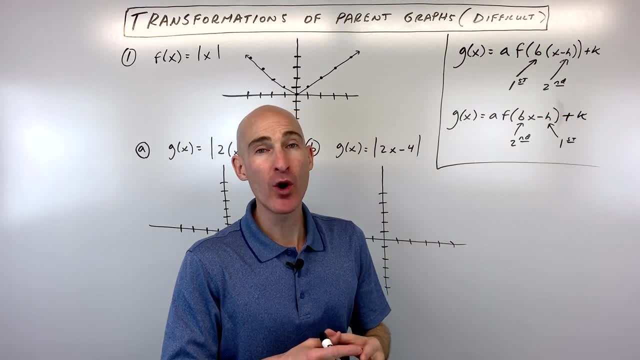 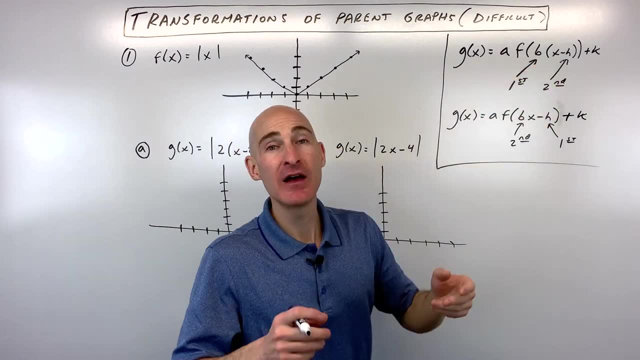 it's going to shift. Whereas with the b, if like b is greater than one- like, say, for example, two- it would actually divide all the x coordinates by two. If it was like a half, it would actually multiply the x coordinates by two. So it has the opposite effect, it has the reciprocal effect. 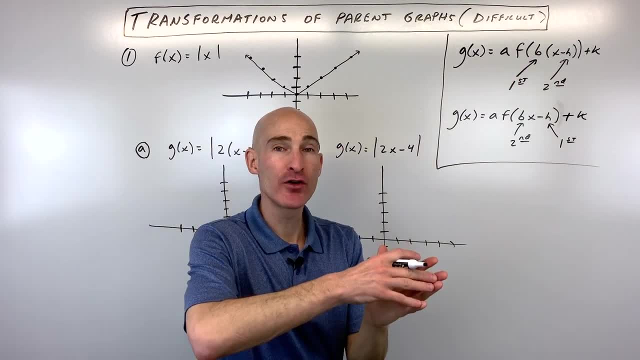 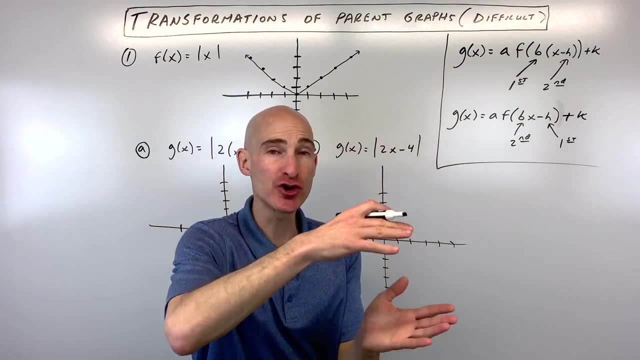 this b value, And then here this coefficient a. this is our vertical stretch or compress. If a is greater than one, it's a vertical stretch. If it's between zero and one, it's going to be a vertical shrink or a vertical compress, And if it's negative, it's going to reflect over the x. 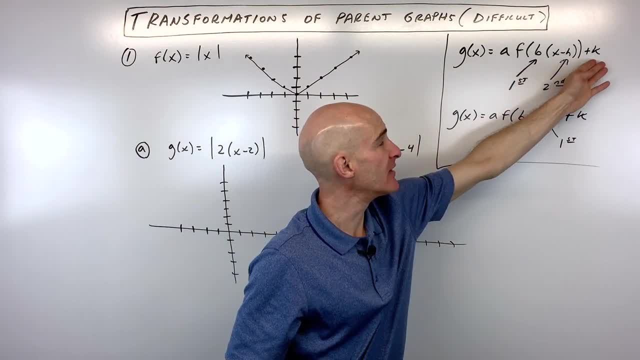 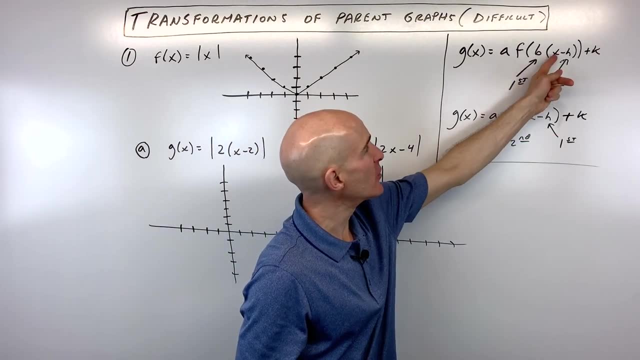 axis, So it's a reflection if it's negative. And then, lastly, the k that's going to be our vertical shift up and down. Now, if it's in this form here, what you can see is that this b value is like distributed in, it's not factored out. And so, when it's in this form, what you want to, 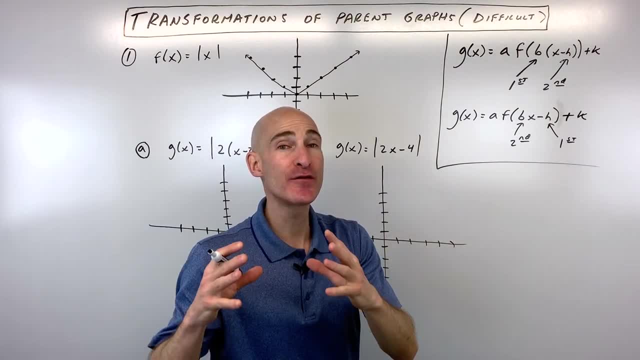 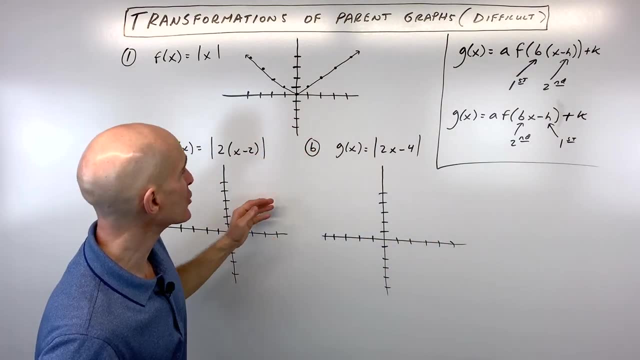 do? is you actually want to do the horizontal shift first and then follow that up? So it's it by the horizontal stretch or compress. We're going to go through a number of examples. I'll show you how this works. The first example we're going to work with is the absolute value function. 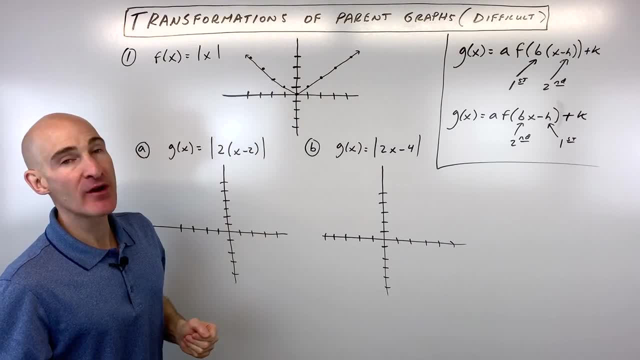 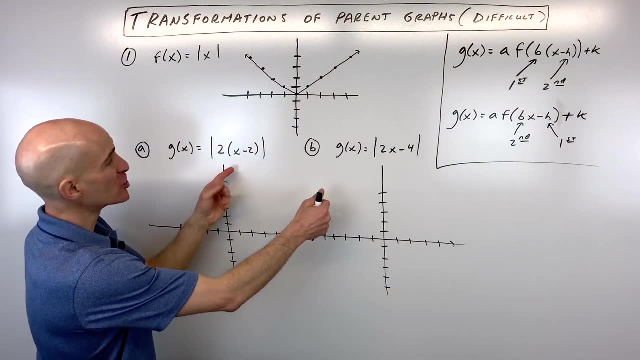 and you're familiar with this graph already. It's a v-shaped graph. If you're not familiar, just go ahead and make a table, pick some negative values- 0, and some positive values, and you're going to get that v-shaped graph. But what I want to compare and show you is the difference between: 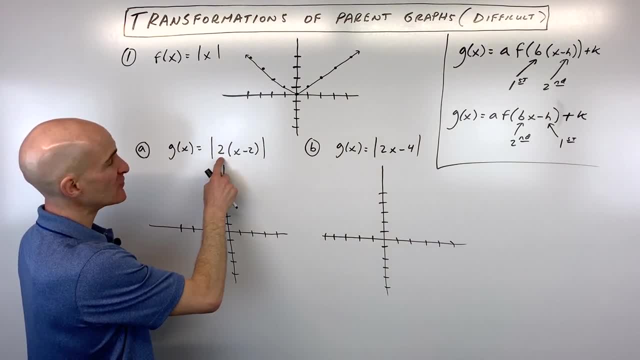 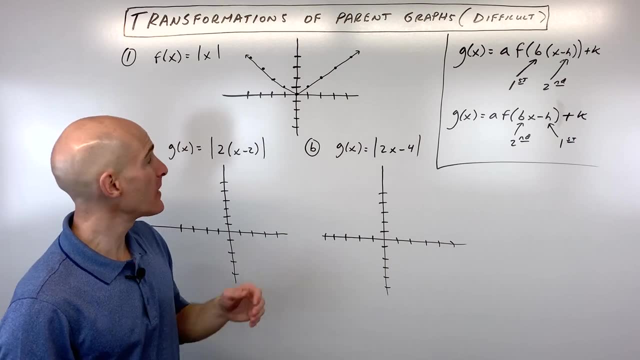 graphing it in this form, g of x equals the absolute value of 2 times x minus 2, and g of x equals the absolute value of the quantity 2x minus 4.. Now you might be saying: Mario, these are exactly the same, right? If I distribute the 2, that's 2x minus 4, which is exactly what we have. 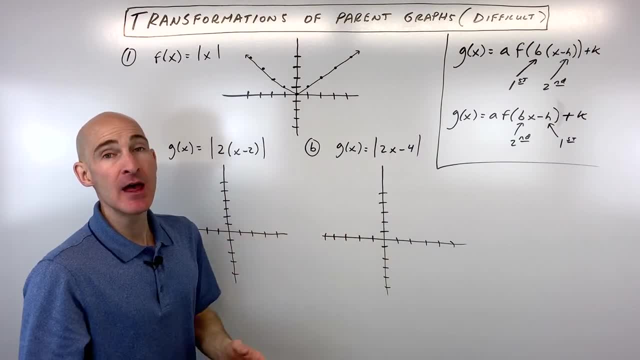 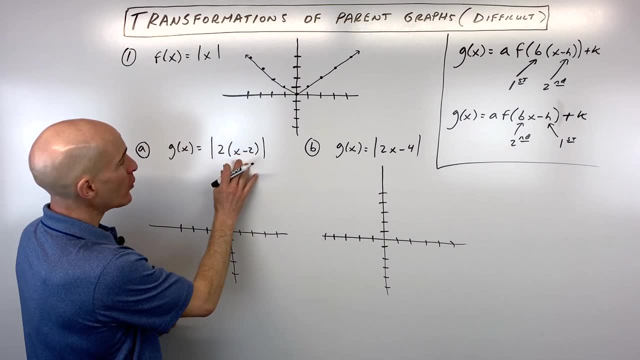 here and you'd be exactly right and we're going to end up with the exact same graph. But when you describe the transformations, the actual steps that you go through are going to be different. So let me see if I can explain So in this form, you can see that that 2 is factored out, So when it's 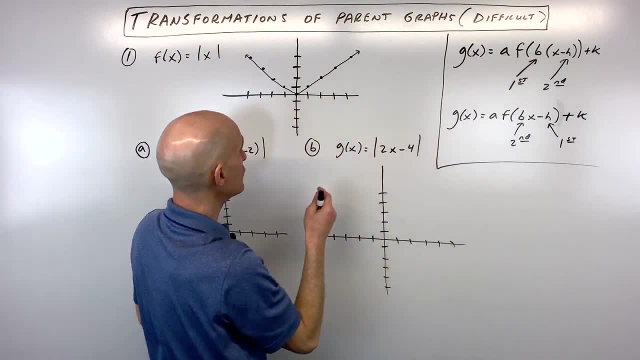 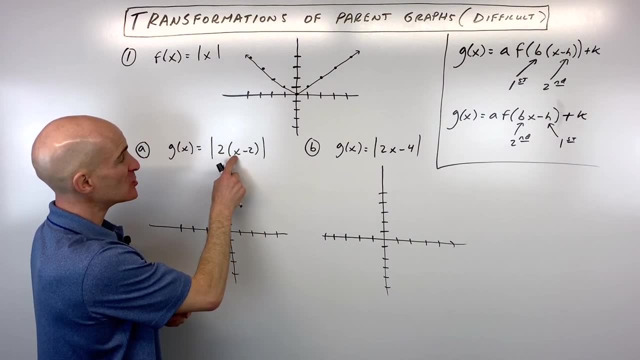 factored out. it's in this form here, which means that we actually want to take the horizontal stretch or compress into account First. so what we're going to do is we're not actually going to multiply the x values by 2. This has the opposite effect. we're going to divide the x values by 2.. So it's going to be a 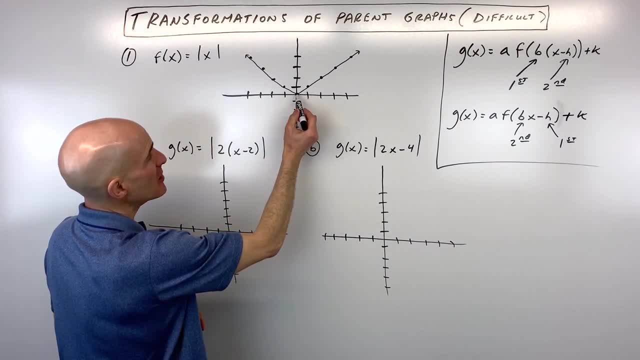 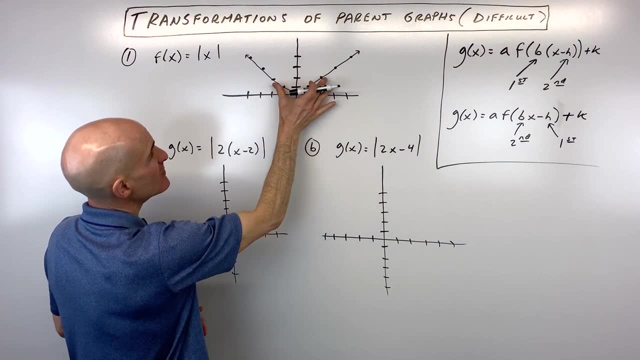 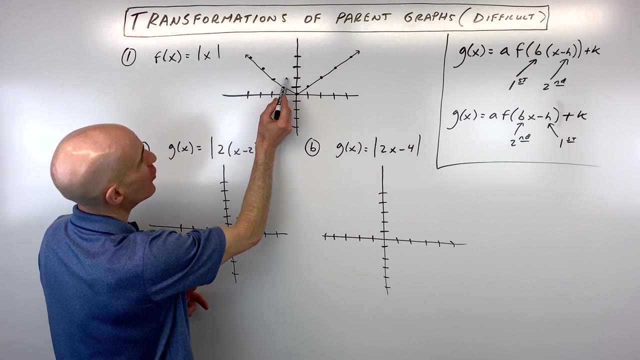 horizontal shrink. So what that means now is this point here is going to stay exactly where it's at, but this point here- see how the x coordinate is 2? It's going to be shrinking, so that means that this point is actually going to be at 1. now Same thing over here. see how this is at negative 2?. 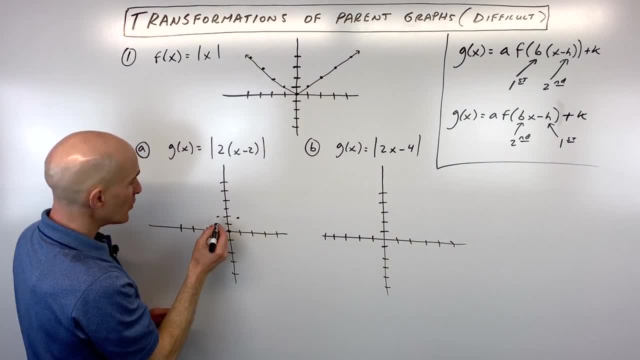 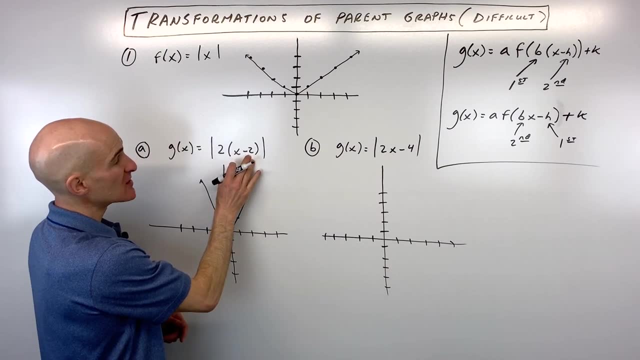 A horizontal shrink. this is going to put this at negative 1.. So what you can see here is we've got a graph that's been horizontally compressed. Then what we're going to do is we're going to do this part second the h value. So we're going to say this is going to shift, not 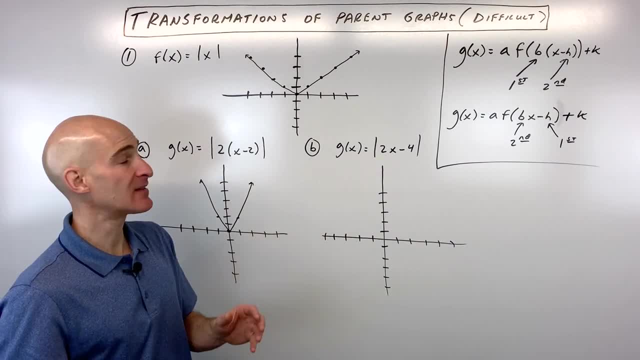 minus 2, not left 2.. It has the opposite effect. when it's a group of the x like that, It's actually going to shift right 2.. So each of these points, I'm just going to go right 2.. This point over here. 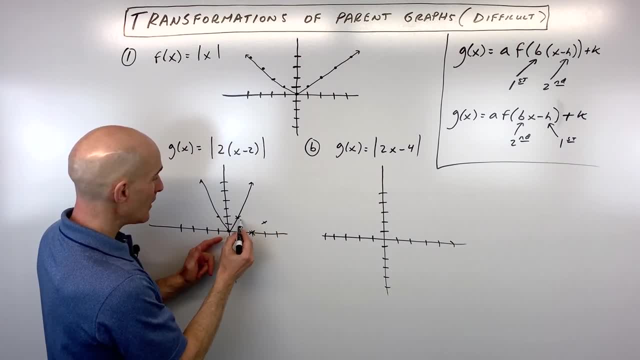 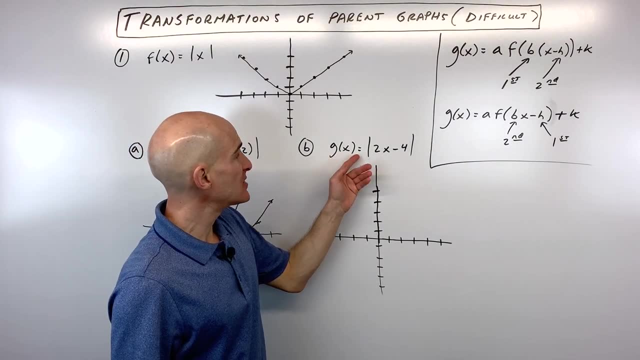 right 2.. This point over here, right 2.. And so you can see that's our final graph, right there. Okay, now let's take a look at letter b. g of x Equals the absolute value of 2x minus 4.. Notice now that the 2 is not factored out. This is all. 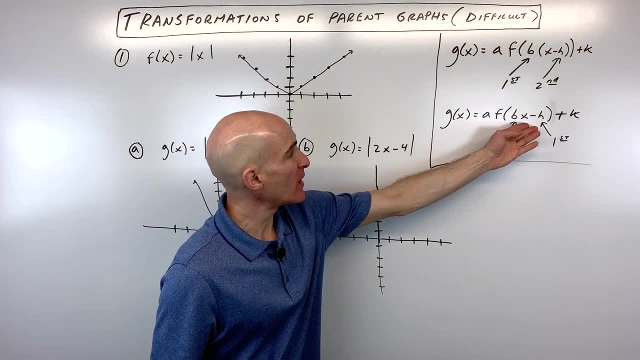 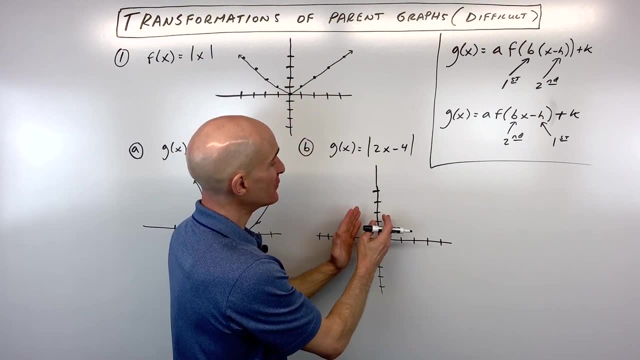 you know, multiplied together here What we want to do is in this form: right here is we actually want to do the horizontal shift first. So the minus 4 actually tells us this graph here is going to be shifted right 4.. So this vertex here is now going to be at 1,, 2,, 3,, 4, right here. 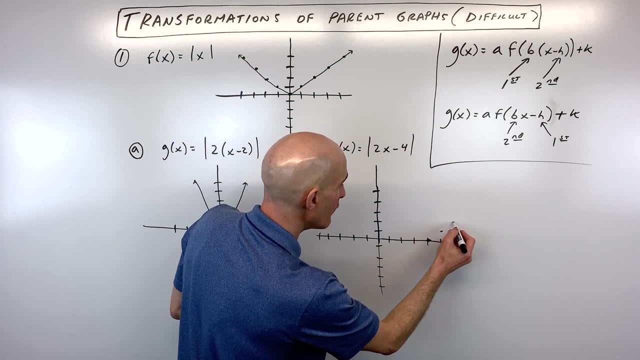 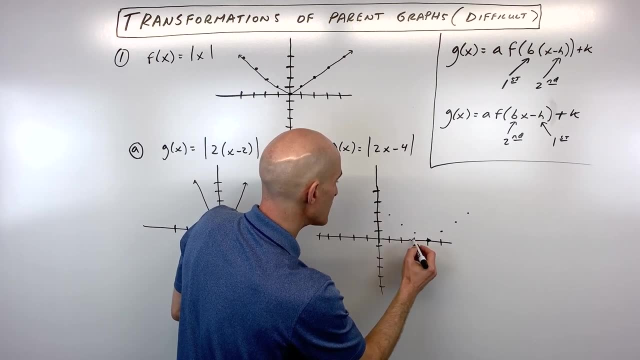 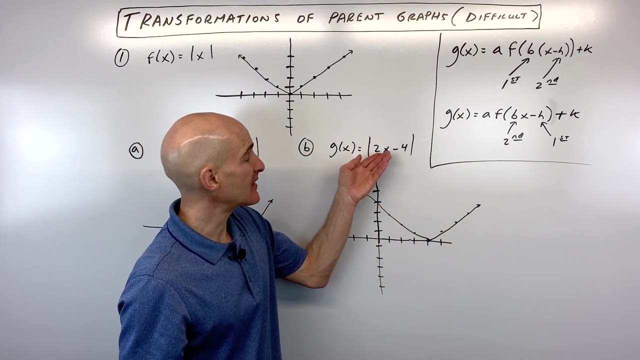 And you can see. then it's going up with a slope of 1.. Okay, like this same thing over here. Okay, so that's our shifting right. 4.. Okay, now the 2 we want to take into account. Remember, this has the opposite effect on the graph. This is actually not going to multiply the x values by 2, but 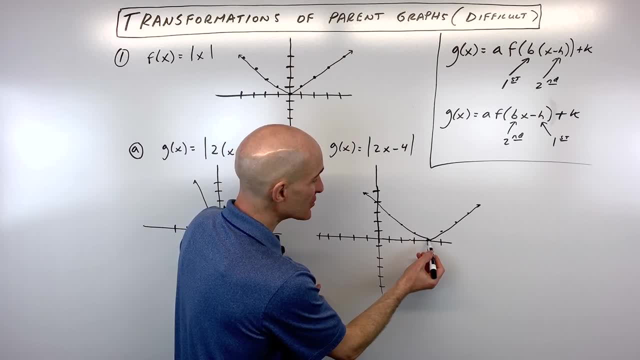 actually divide the x coordinates by 2.. So this point here, instead of being at 4, is now going to be at 2.. Okay, this point over here which is at 0 is 0. divided by 2 is still 0. So that's going to. 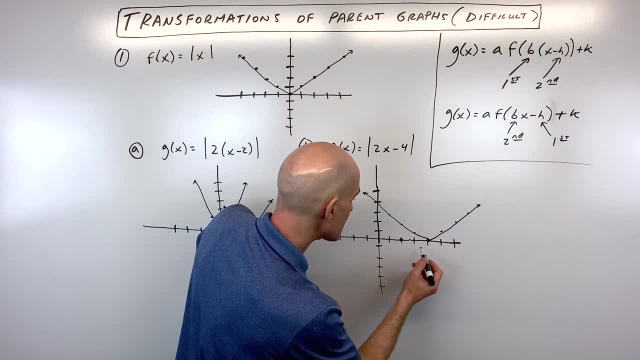 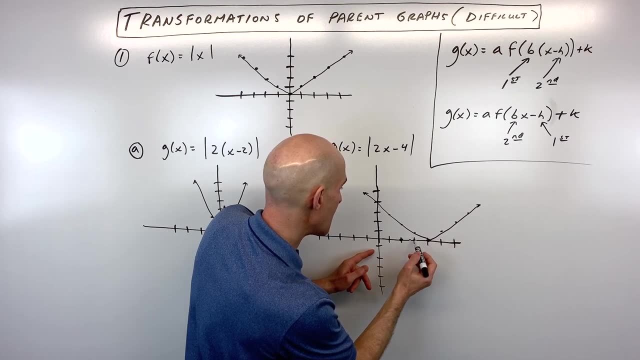 stay exactly where it's at. And then take, for example, another point here. Let's say this is 1, 2, 3, 4, 5, 6 comma 2.. It's a little bit high here. This is actually going to be at 3. 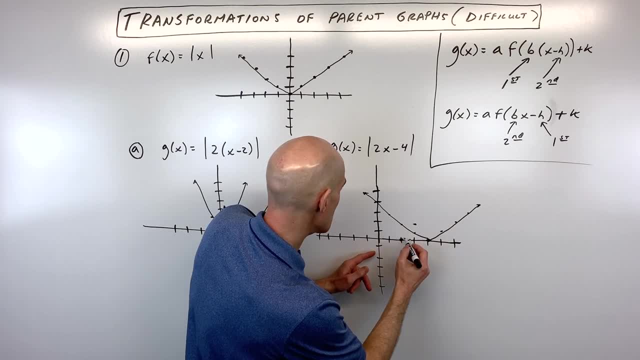 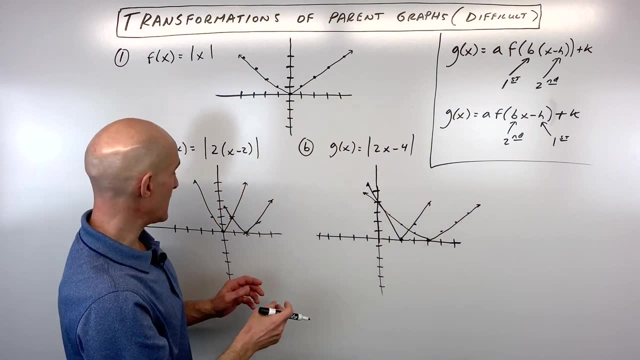 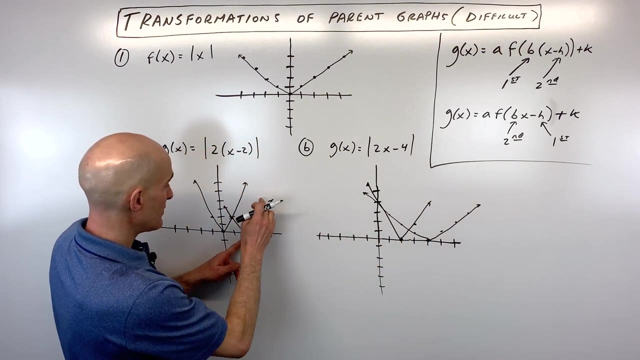 comma 2, which is right there. So you can see now that the graph is actually going to look like this and if you look closely, these two graphs are exactly the same. See how we're at: vertex is at 2 and it's going up like so. Same thing here: it's: vertex is at 2 and it's going. 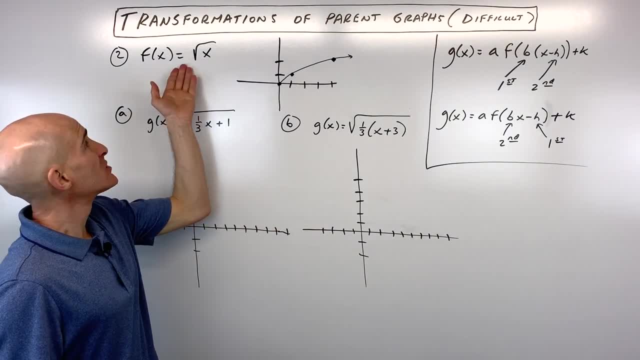 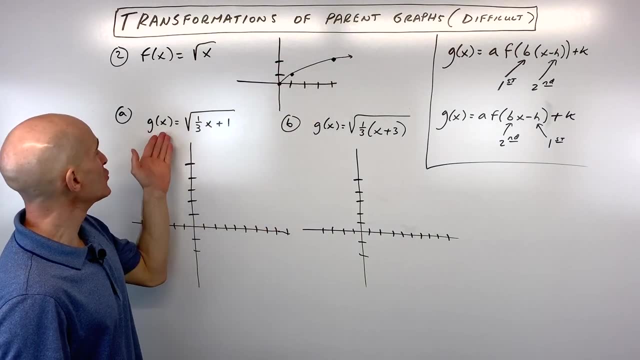 up at the same rate. Okay, example number two: we're going to work with the square root function, and you know what the shape of that graph looks like. it's kind of like a parabola on its side, just the top half there. So what we're going to do is letter a and letter b. again, look at these two functions. 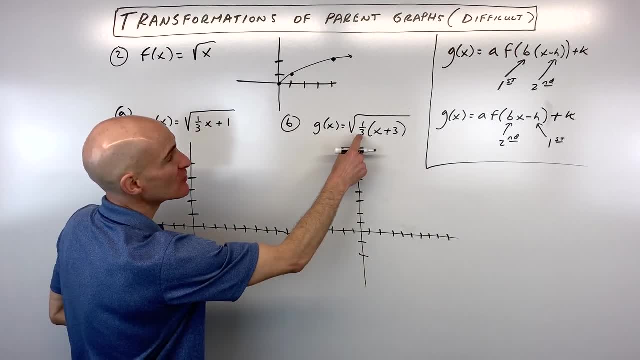 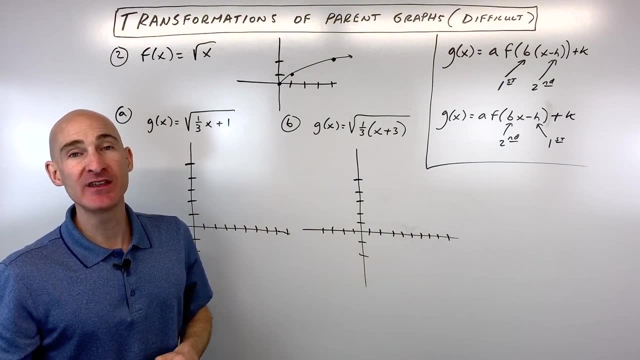 you might say to yourself: well Mario, it looks like they're exactly the same. if I distribute this one-third, I'm getting one-third x plus one, the same as example a here. but the process of graphing these, the process of describing the transformations, is going to be different for both of these. 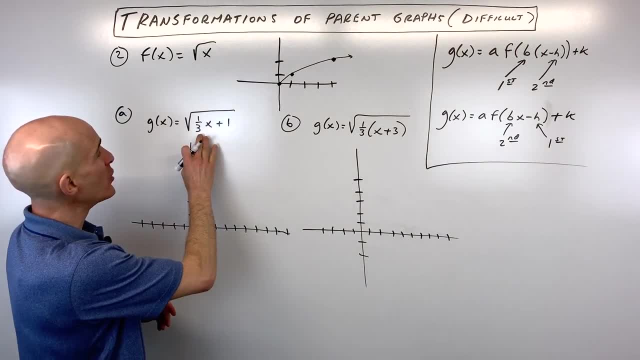 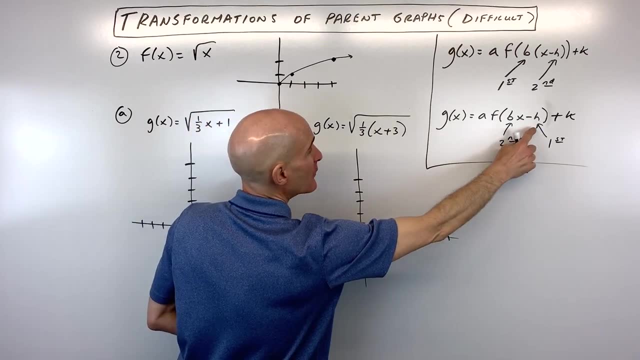 So let me show you how you would work these. so for this one, notice that the b-value is not factored out. so that means it's in this form here, and when it's in this form, what we have to do is do our horizontal shift first. so this plus one is actually going to take this. 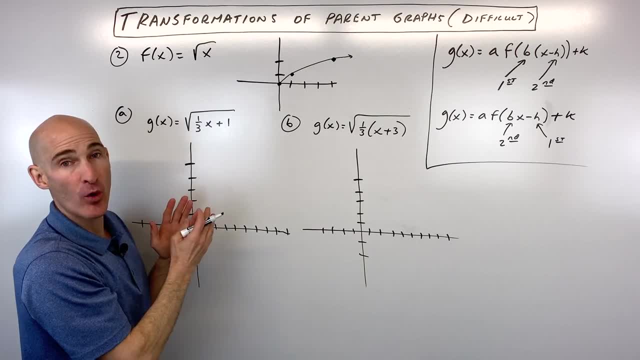 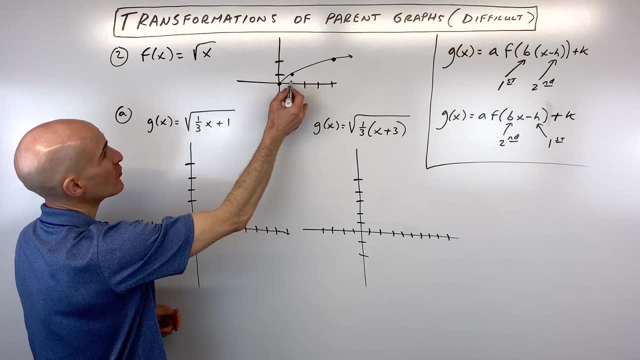 graph here and it's going to shift all the x coordinates left one. so instead of being here at zero-zero, we're going to be over here at negative one. instead of being over here, we're going to shift to left one. we're going to be right there instead of being at four. 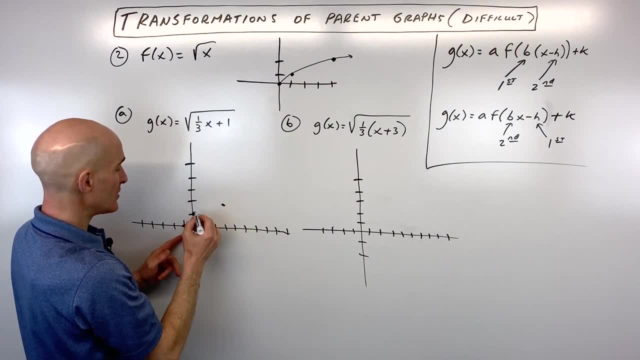 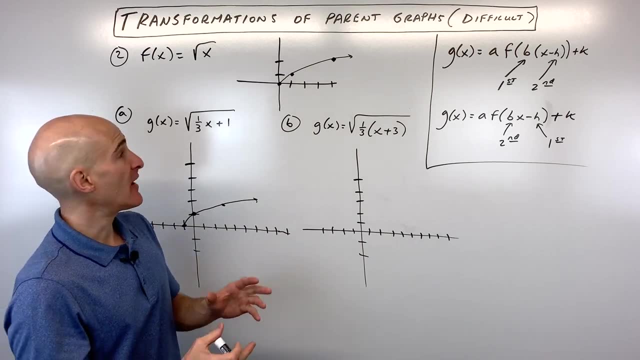 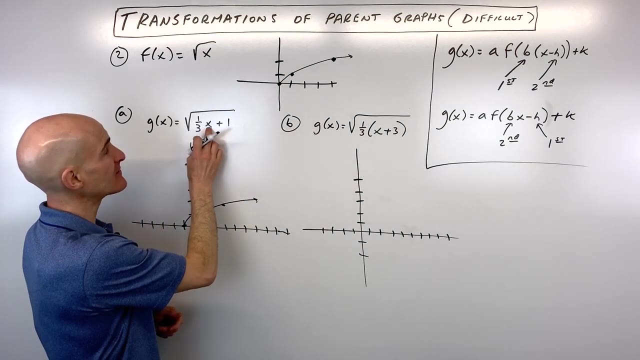 two. we're going to be at three. two, So everything just shifted left. one. Okay, now the one third. this is going to have an effect on the horizontal stretch or compress, but remember, this actually has the reciprocal effect. So it looks like you're dividing the x values by three. You're actually 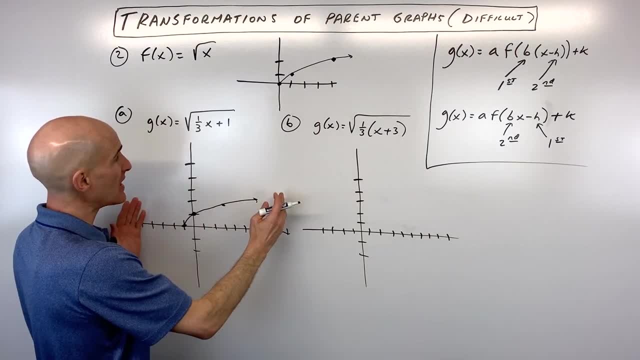 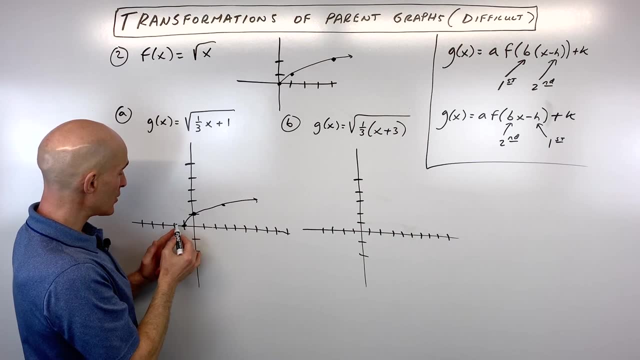 going to be multiplying the x values by three. So this is actually a horizontal stretch. So what I'm going to do is I'm going to take all the x values and multiply them by three. So instead of being at negative one here, we're going to be at negative three right here, Instead of being at zero. 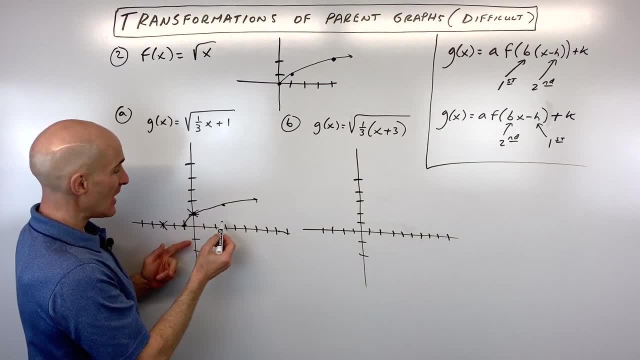 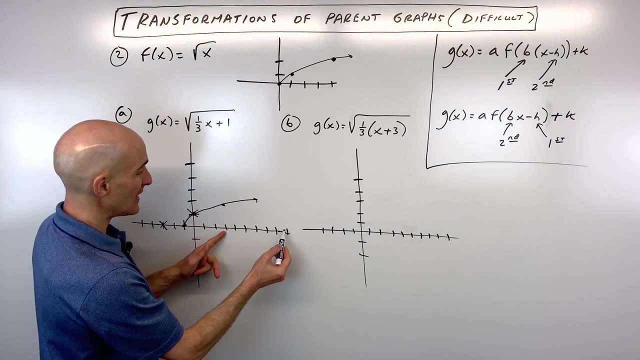 well, zero times three is still going to be zero, So that stays where it's at. and then this one over here: instead of being at positive three, you're going to be at positive nine. So four, five, six, seven, eight, nine, and the y value is going to stay the same though. Okay, so we're just changing the 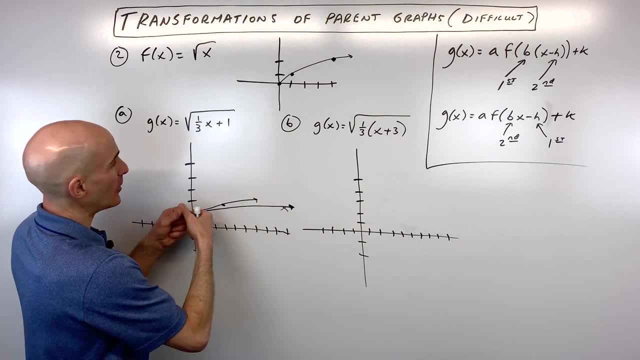 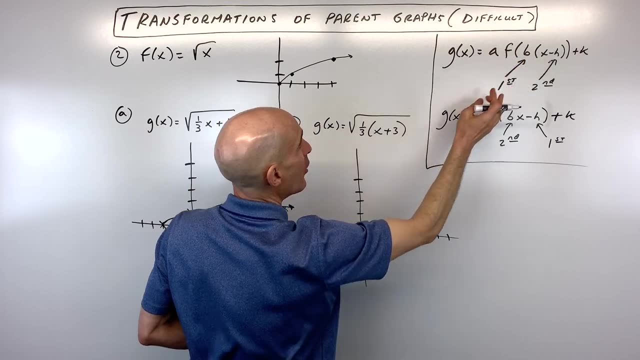 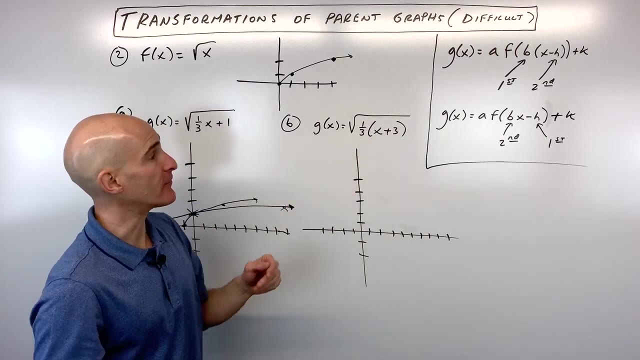 the x coordinates and you can see this is a horizontal stretch. Okay, now for letter b. you can see that this B value has been factored out, And so what that tells us is that we actually have to do the horizontal stretch or compress first, Followed by the horizontal shift. So what does the 1- 3rd do? Well, again, just like we talked about over here. 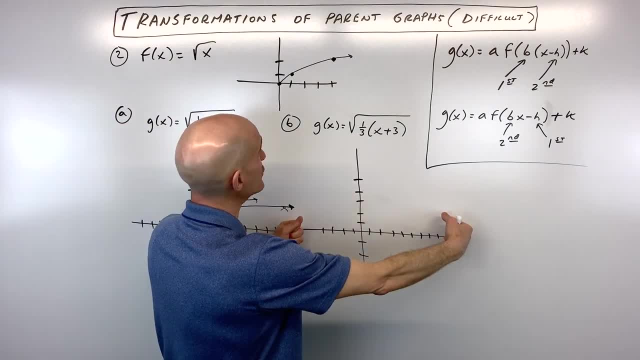 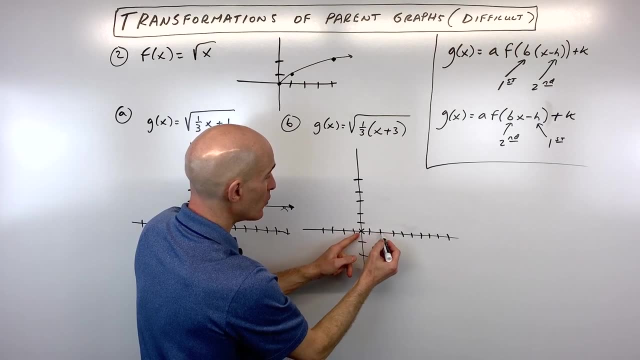 It's going to have the reciprocal effect. It's actually going to multiply the x values by 3. 0 times 3 is still going to be 0. 1 times 3 is going to be 3. so 1, 2, 3 again, the y value stays the same and over here. 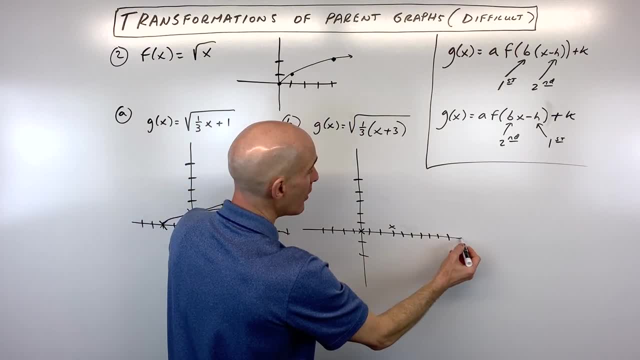 We're at 4, comma 2.. So now we're going to be at 12, Comma 2.. So this is 1, 2, 3, 4, 5, 6, 7, 8, 9, 10, 11, 12. 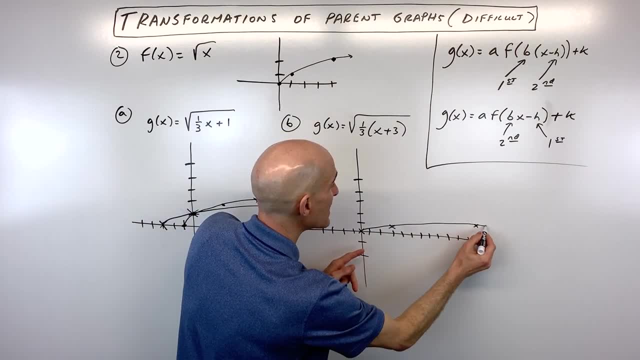 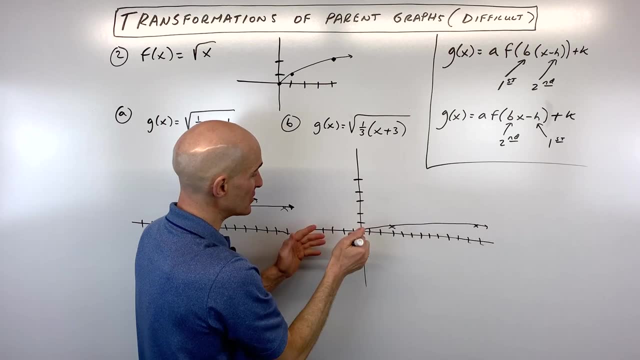 Comma 2 right about there. So you can see we did the horizontal Stretch first. now all the values are going to be shifted: not positive 3, but the opposite left 3. So this point is going to be 1, 2, 3. right here. This point is going to be: 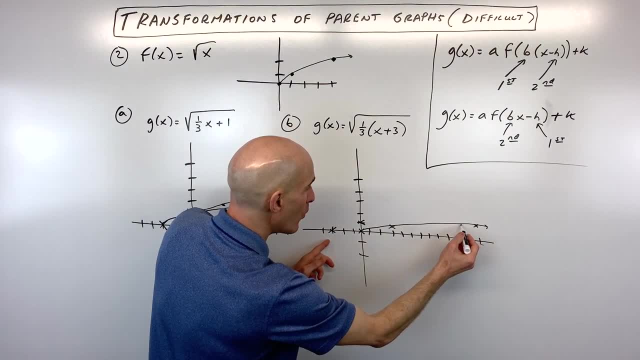 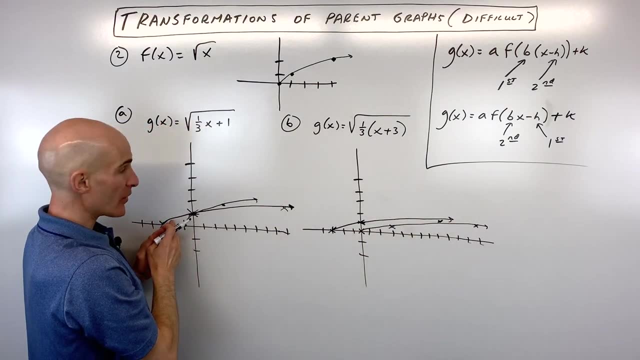 1, 2, 3 right here, and this point is going to be at 1, 2, 3, Right about there. What you can see is we're getting the exact same Graph. it's just that the process of getting to that graph was a little bit different. the order of the transformations was different. 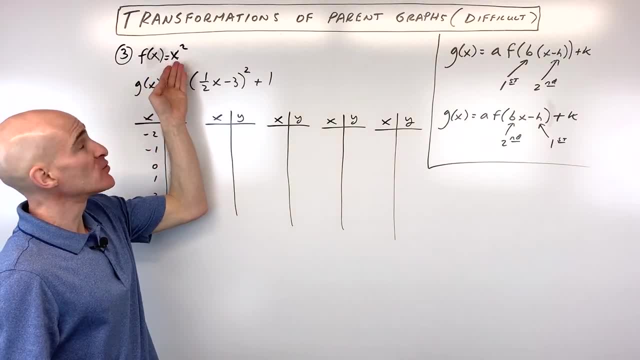 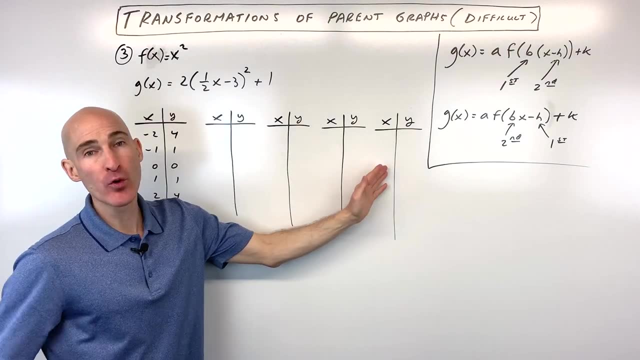 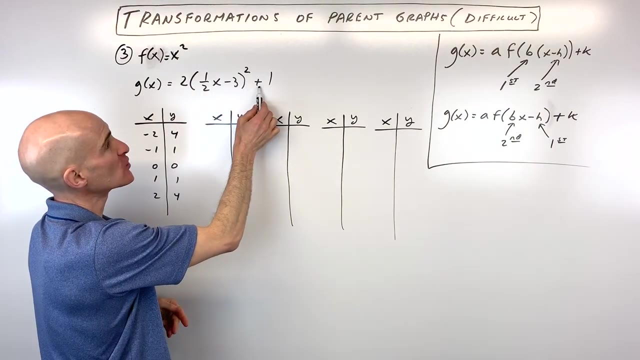 Okay, example 3: We're going to work with. f of x equals x squared. This is the parabola graph that you're familiar with, but what I want to show you now is how to use a table to get the final coordinates of. You know your new function here: g of x. so g of x equals 2 times 1, half x minus 3, the quantity squared. 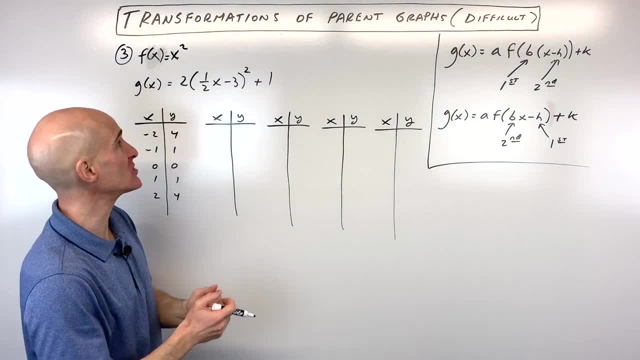 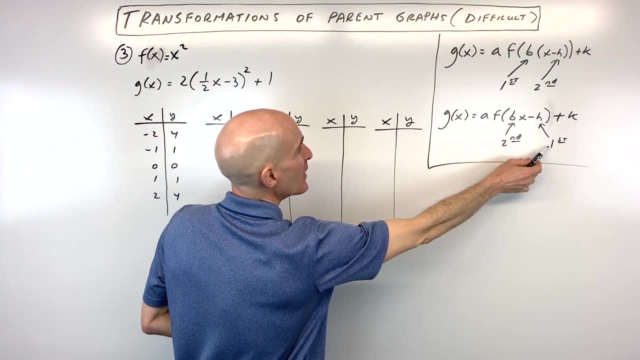 Plus 1. so the question is, is what do we do first? as far as transformations, Well, you can see that we don't have that b-value factored out. It's actually just like this form here. So what that tells us is that we have to do our horizontal shift first. 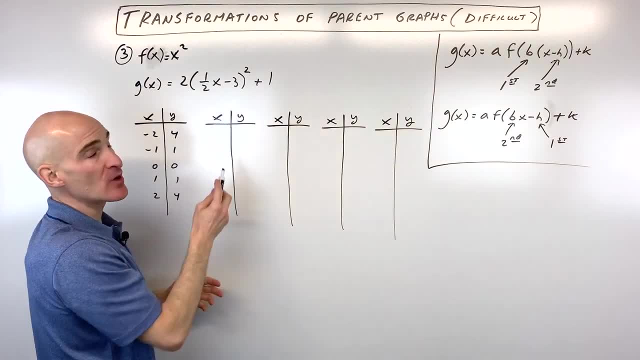 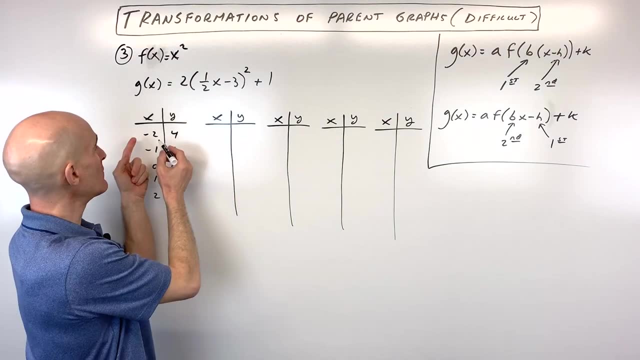 So you can see, our b-value is 3 minus 3. actually is going to take this graph is going to shift it right: 3, Which means that we're adding 3 to the x coordinates. So what I'm going to do is- I just took these: 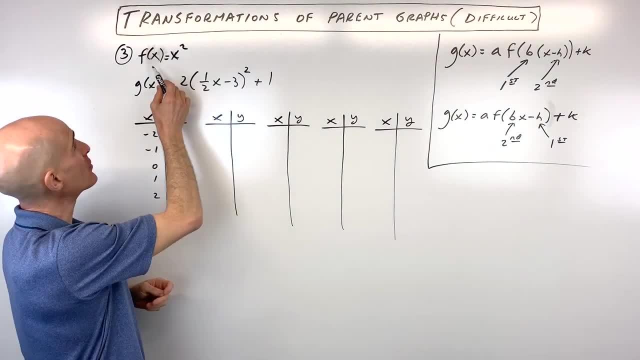 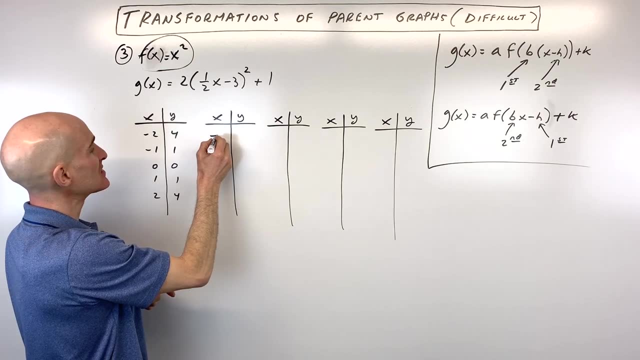 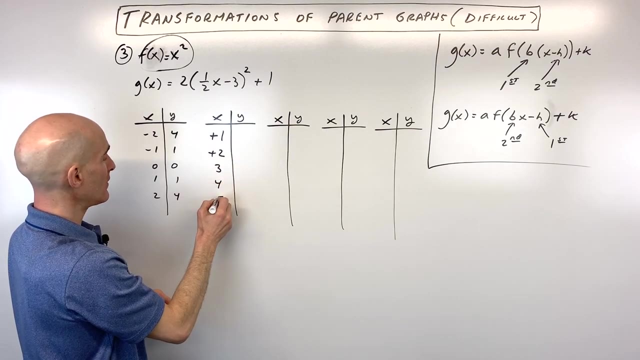 Parent function coordinates here: negative 2, 4, negative 1, 1, etc. just with this equation here, and what I'm going to do now is I'm going to add 3 to the x-coordinate. so that's going to make this Positive 1, that's going to make this positive 2, that's going to make this 3, 4, 5. 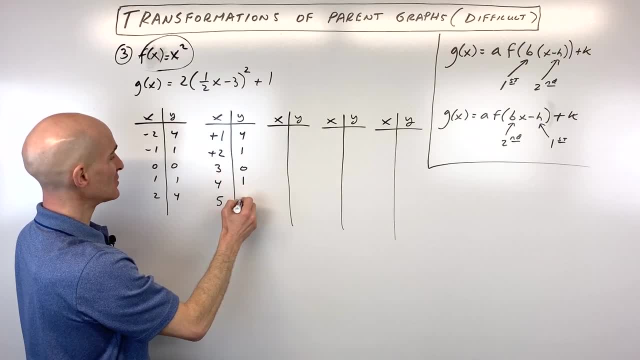 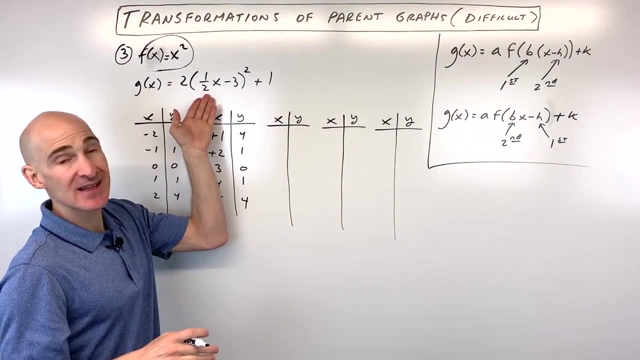 But the y-values are going to stay the same because this is just shifting to the right. 3. Now we're going to do is we're going to focus on the horizontal stretch and compress. This is our b-value, Remember. it has the opposite effect. It looks like you're multiplying by 1 half. You're actually. 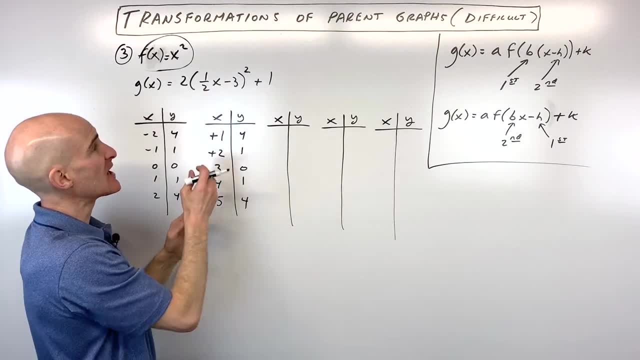 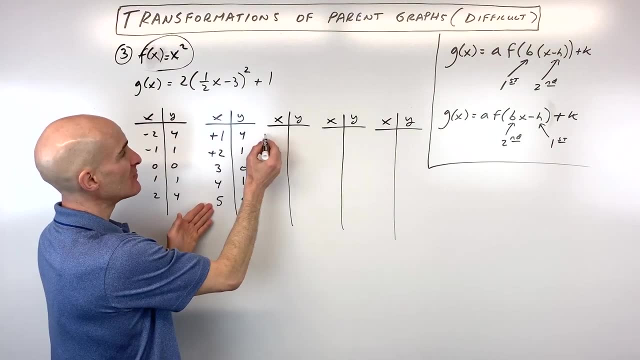 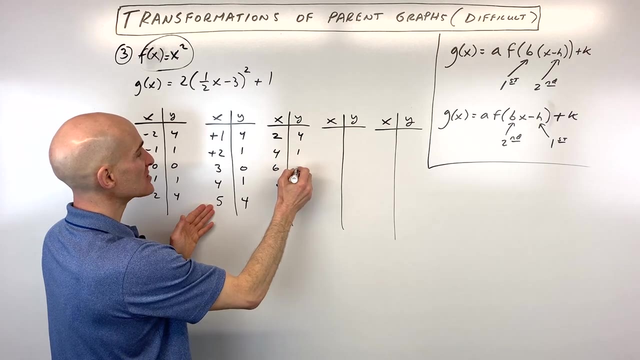 multiplying by the reciprocal 2 over 1. So this is actually going to be a horizontal stretch, Which means that we're multiplying the x-coordinates by 2. so now, instead of being at 1, we're going to be here at 2, 4, 6, 8 and 10, but the y-values are going to stay the same. 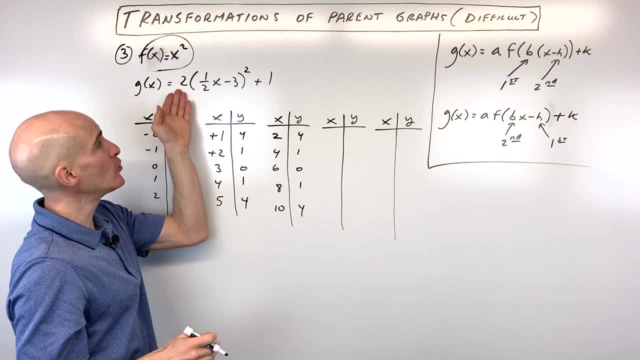 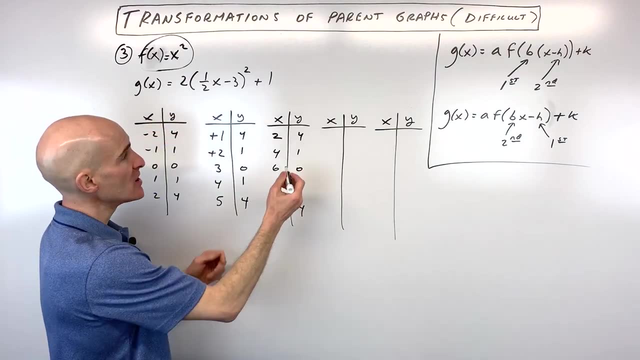 Now we're going to go focus on the a value here. The 2 actually has the effect on the vertical component. It's going to multiply the y-values by 2. It's a vertical stretch, So the x-values are going to stay the same: 2, 4, 6, 8 and 10. 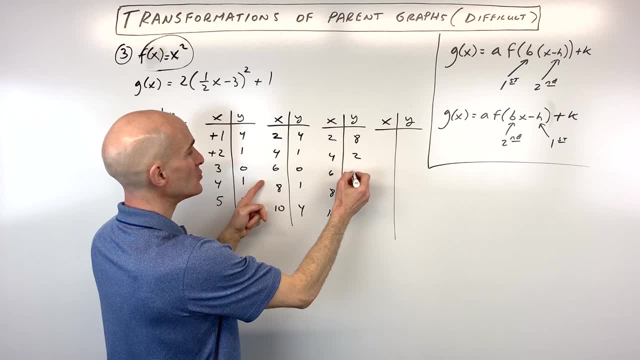 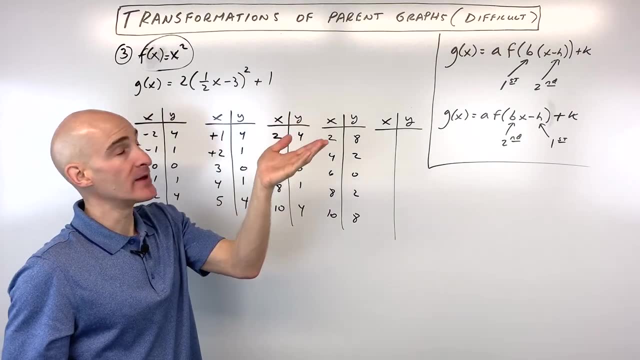 But the y-values are gonna be doubled, so this is going to be 8, 2, 0, 2 and 8. The last thing we want to do is this key value here, Which is going to shift it up one, so it has the same effect if it's positive. one up one. 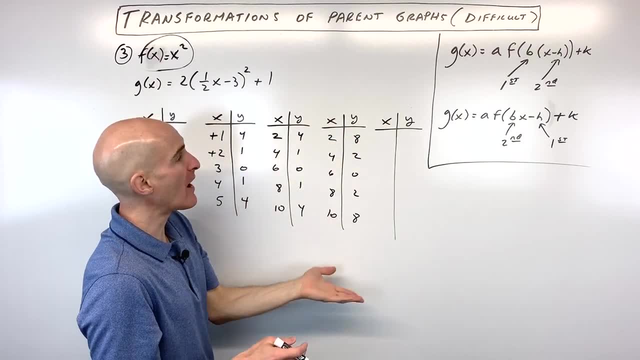 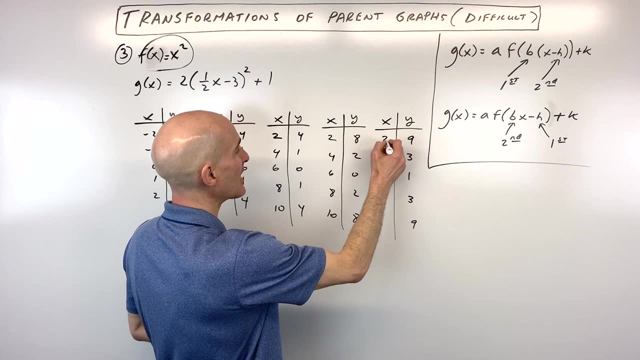 If it was negative, want to go down one. So that means we're going to add 1 to all the y-values, since it's shifting in the vertical direction. so this is going to be 9, 3, 1, 3 and 9, but the x values are going to stay the same: 2. 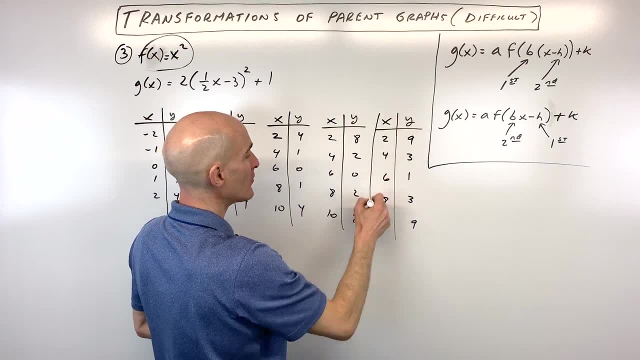 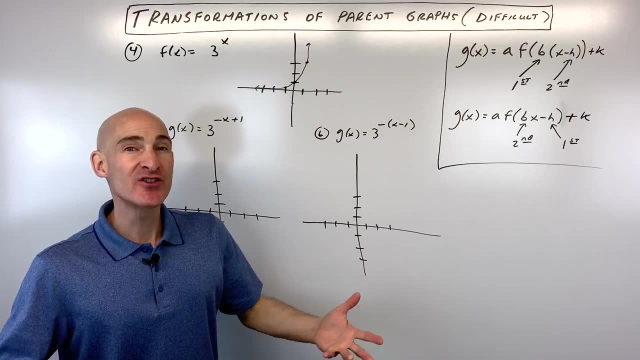 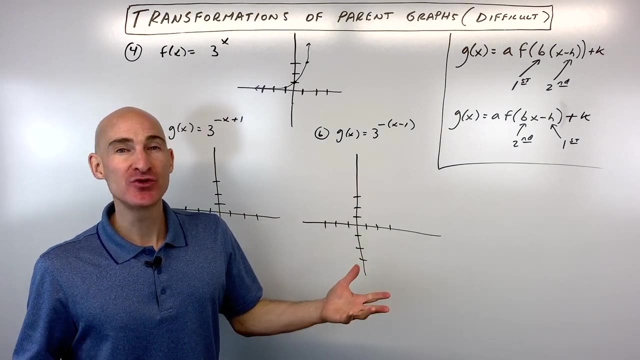 4,, 6,, 8, and 10.. All you have to do now is plot these points and you're going to have your new transformed quadratic function. Okay, so it sounds like you guys are really enjoying this video and, if you like my teaching style, I have a lot more information regarding algebra 2 topics in my 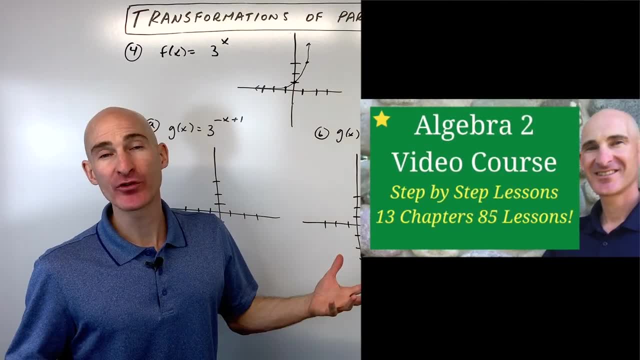 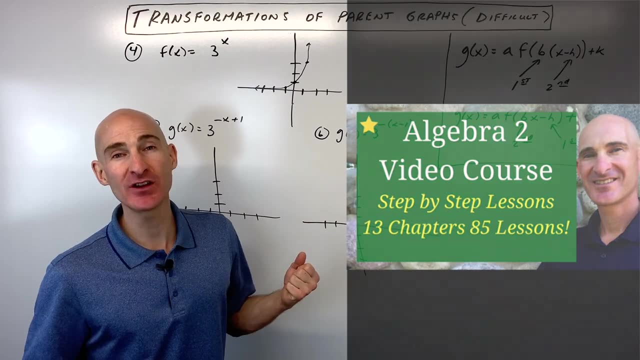 algebra 2 video course. So definitely check that out if you need help with your algebra 2 studies in your class. It goes through a typical algebra 2 curriculum and it goes into a lot of detail, similar to this video but covering all the different topics in algebra 2.. But let's go. 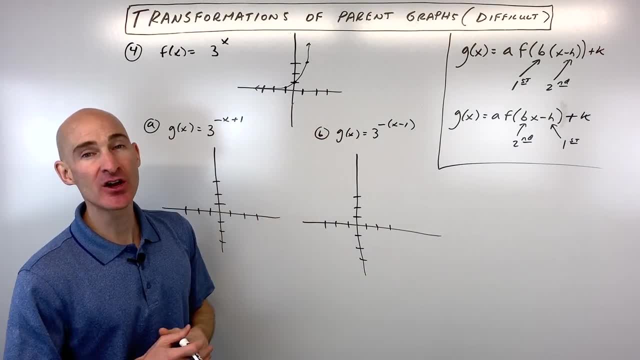 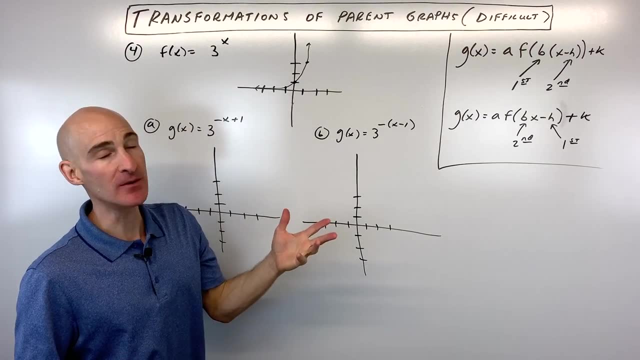 through another example, This one, we're going to be talking about reflections, and this is also one that sometimes confuses students, but here we're working with f of x equals 3 to the x. You can see, this is an exponential growth function. but now we're going to look at two different versions. 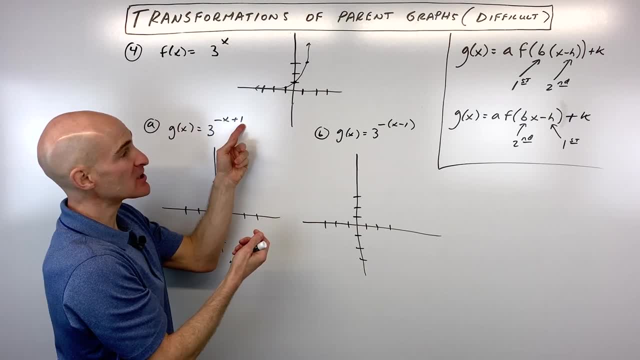 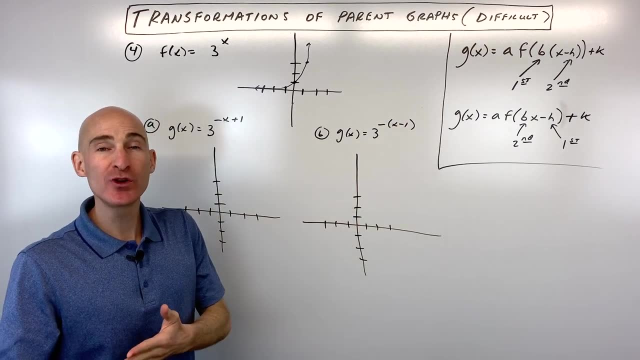 We've got this one, version a, where we have 3 to the negative x plus 1.. Here we have version b, 3 to the negative quantity x minus 1.. So again the question is: what do we do first? What do we do? 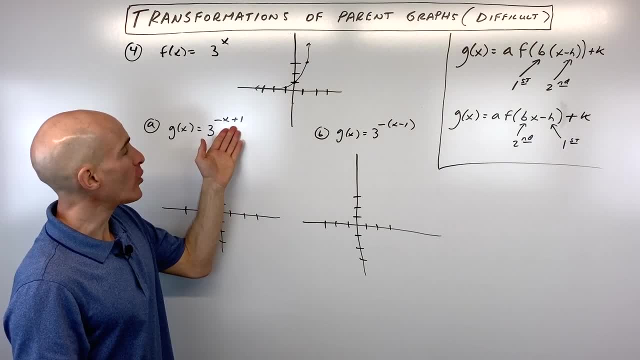 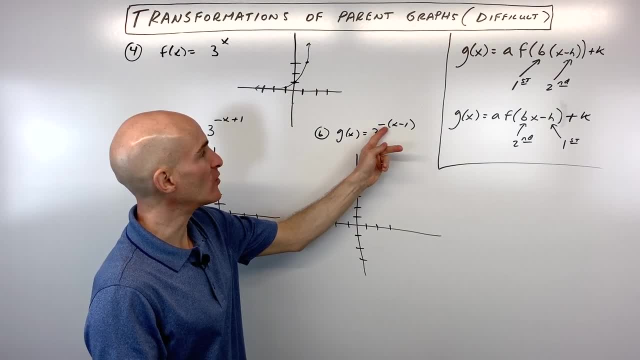 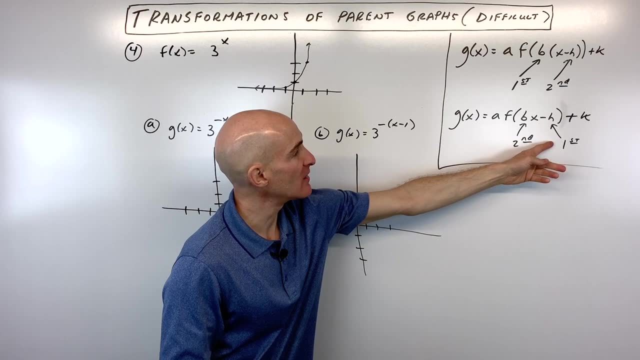 form, you can see that the negative is factored out. Okay, so when it's factored out, that's this form here. This one is not factored out. it's this form here. So what we have to do for the letter a is we actually have to do the shift first. So you can see this plus 1 is actually going to shift. 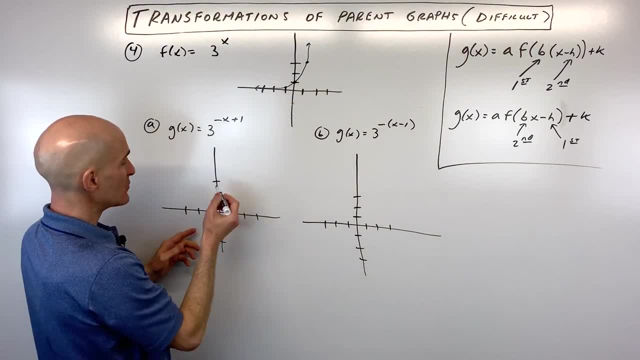 this graph, left 1.. So all these key points here, I'm just going to shift left- 1.. So we're going to go here, This one's going to be over here, And then we're going to shift this one over here. 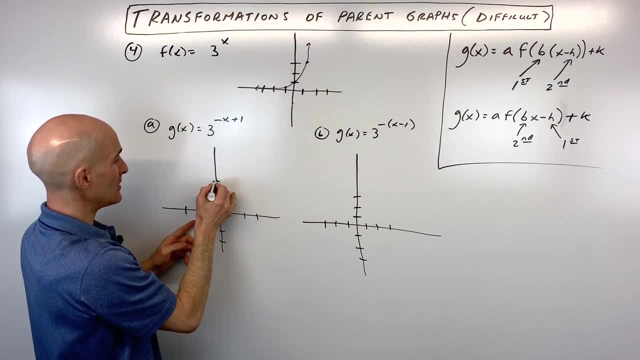 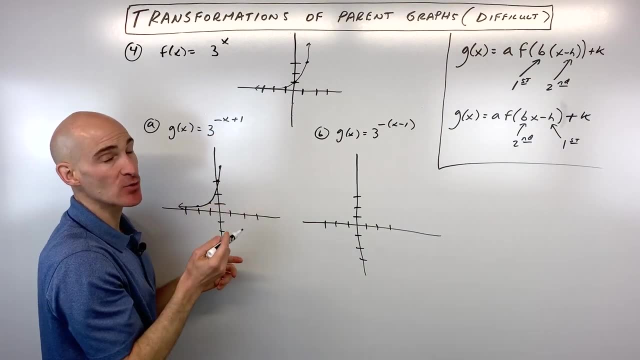 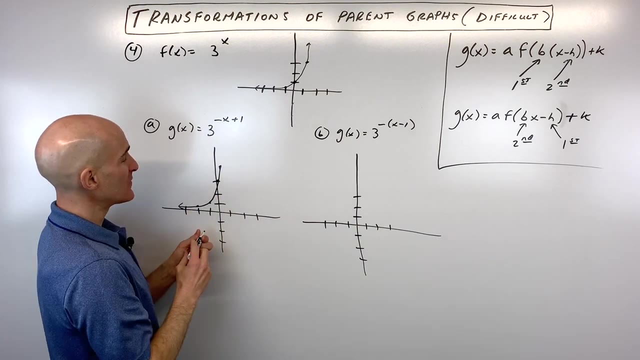 And this one here is going to be right on the y axis. So that's going to be step number 1.. Shifting left: 1.. Now the negative x. what it does is it makes all the x values the opposite, which reflects it over the y axis. So what you can see now is that this point here is going to reflect It's